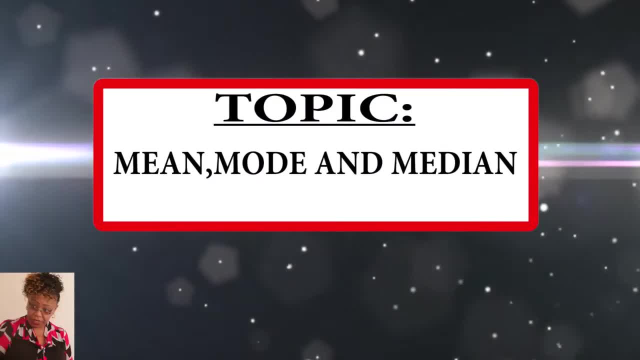 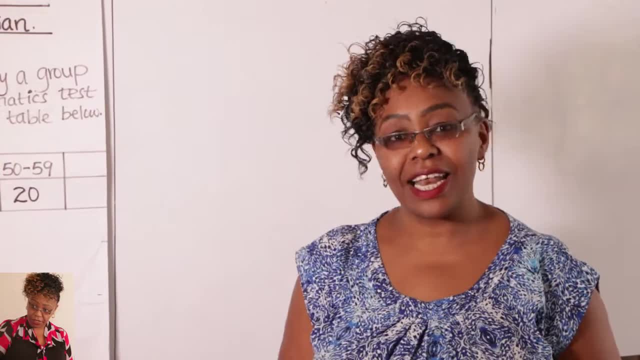 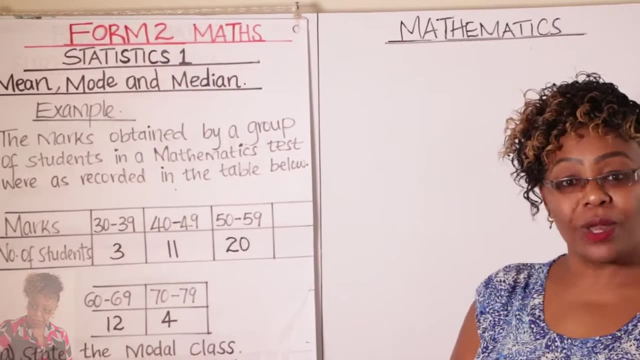 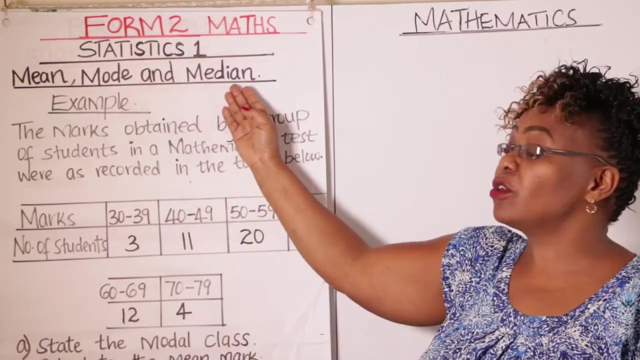 Welcome to my mathematics class. today We are going to look at Form 2 mathematics. Our topic is Statistics 1.. We are going to learn how to calculate the mean, how to find the mode and how to calculate the median of a grouped data. So welcome, my learner, And therefore 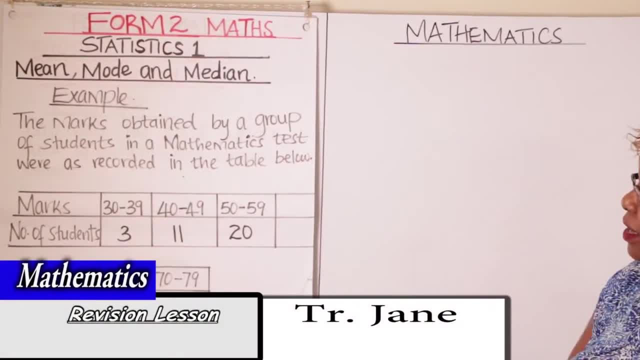 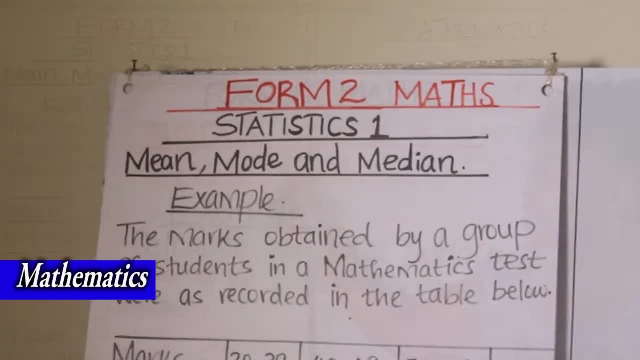 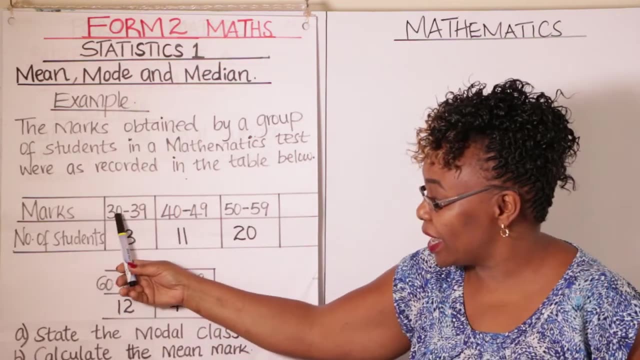 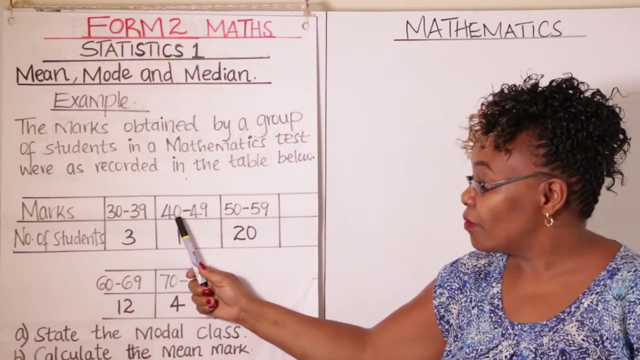 we go straight away to our first question. The question is: the maths obtained by a group of students in a mathematics test were recorded in the table below. So you have the maths of students who got that. There were 3. 40 to 49,. there were 11. 50 to 59,, 20. 60 to 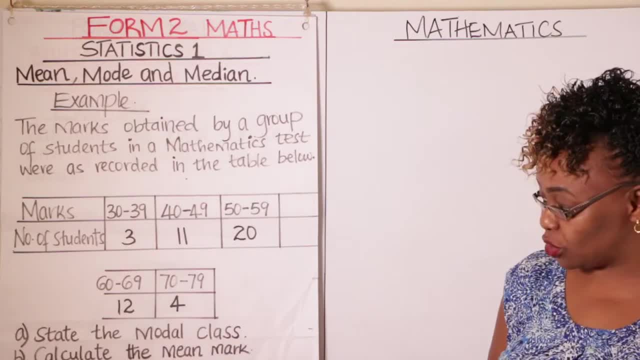 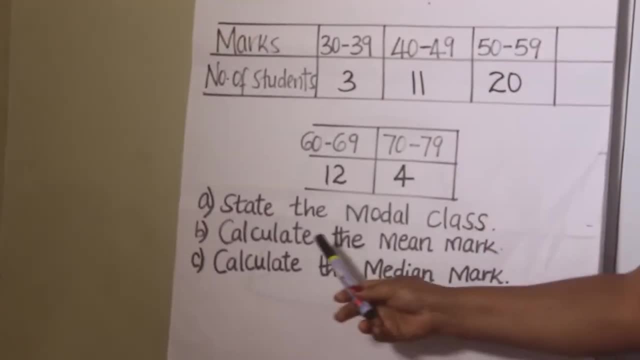 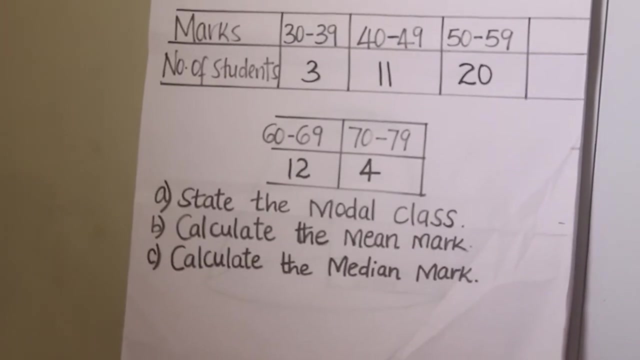 69,, 12.. 70 to 79,, 4 students And therefore our question is: A state the model class. State the model class, Calculate the mean mark And finally, calculate the median mark. Calculate the median mark. So part A, 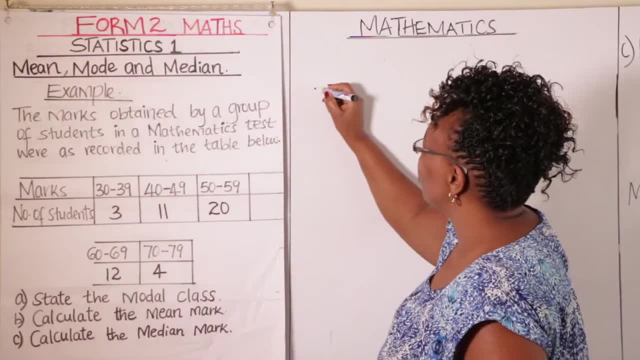 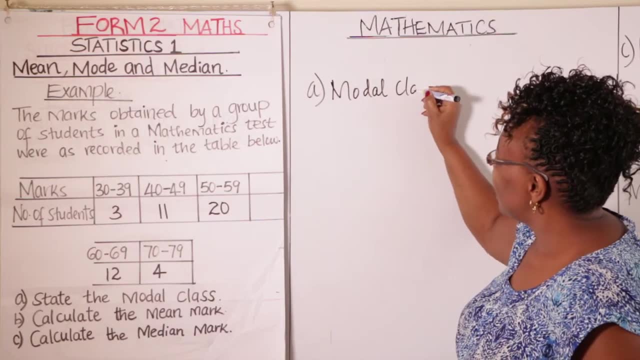 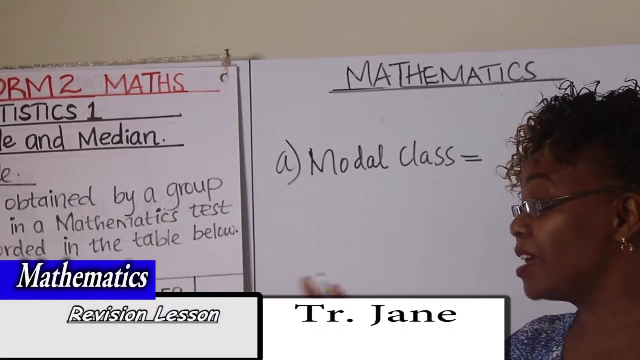 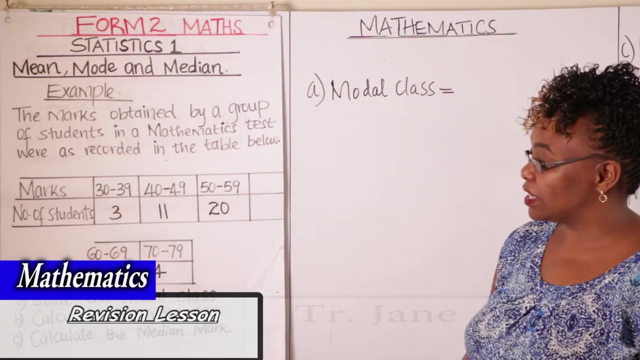 A state: the model class State. the model class State: the model class Model class, learner. Model class Model class refers to the class, to that class which has the highest frequency, to that class where you have majority of the learners, majority of the students. 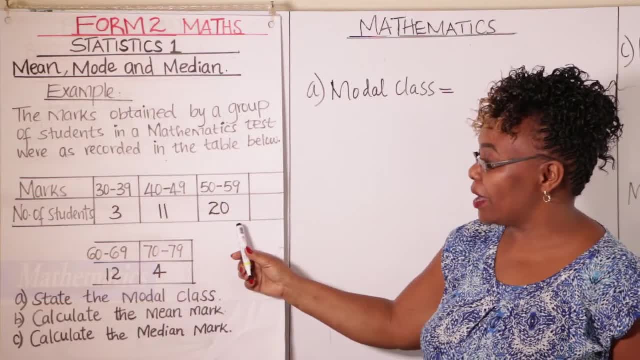 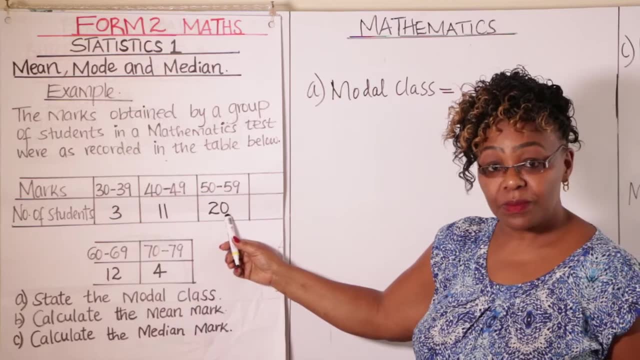 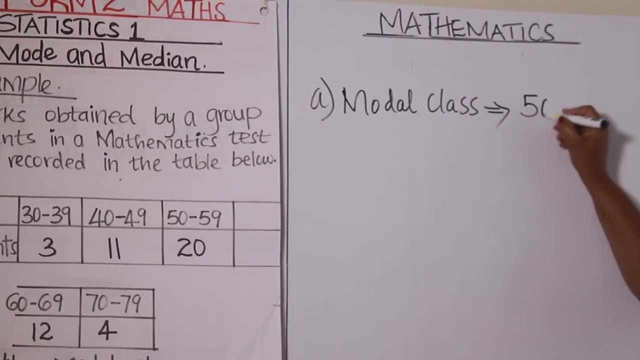 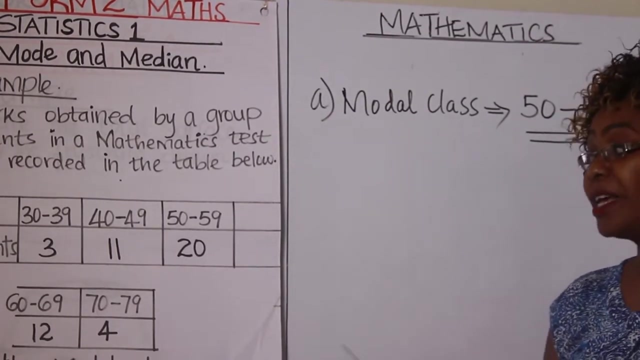 So if you come to our table here, you can see that This class, here this one- 50 to 59,- its frequency is 20.. It has the highest frequency, 20.. And therefore our model class will be 50 to 59. The class which has the highest number. 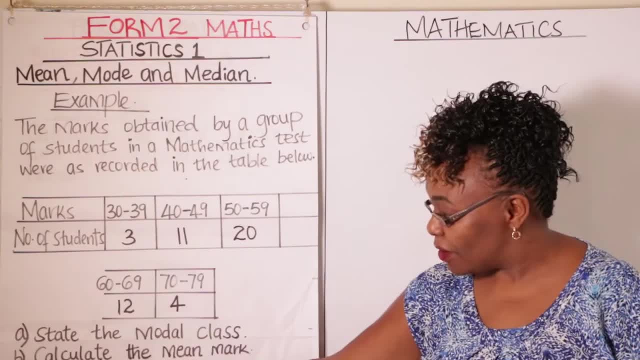 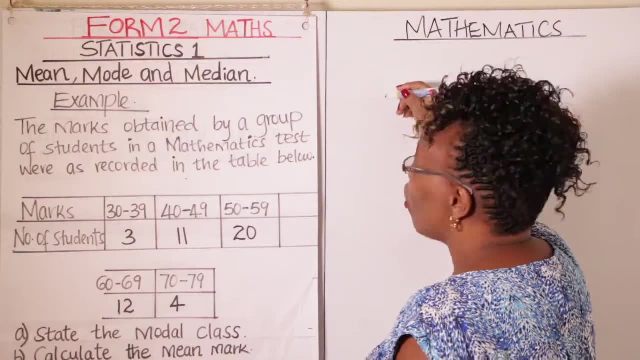 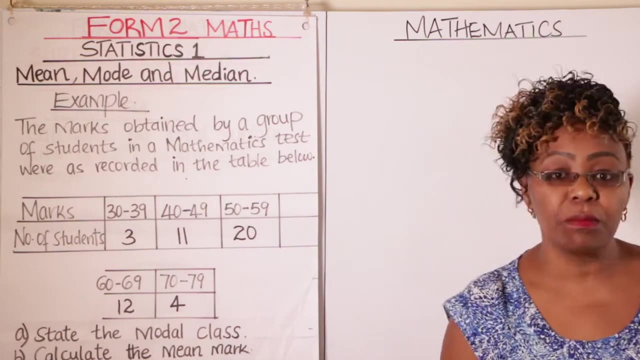 of students And therefore our question is: calculate the mean mark? How do you find the mean learner? And therefore the answer is really simple. You come and draw what we call a frequency distribution table. You draw what we call a frequency distribution table. Let us draw. 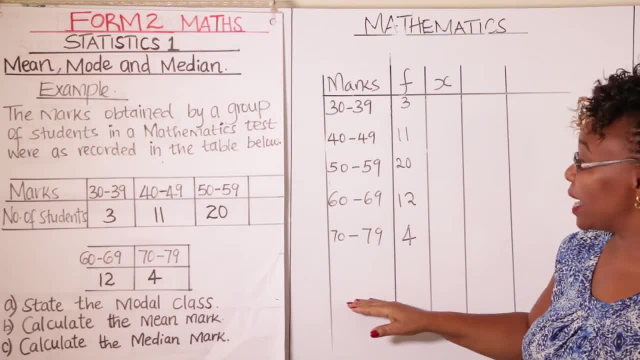 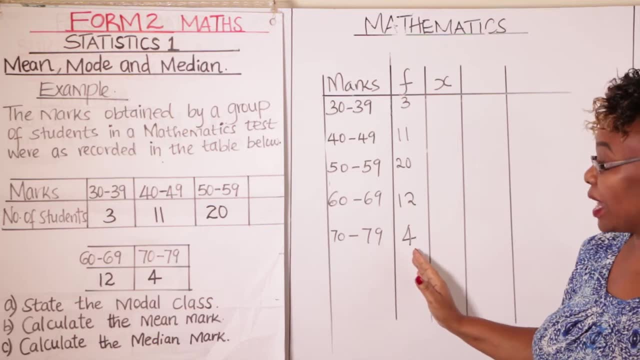 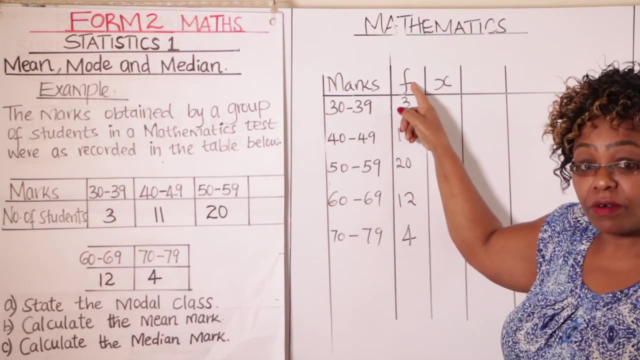 it. You put your classes here or the groups of maths. You put the number of students in the second column. here, You put the number of students in the second column and we refer ability to the number of students as frequency. That is why I've used it, the symbol これ Lo podemos использовать圧 for frequency. 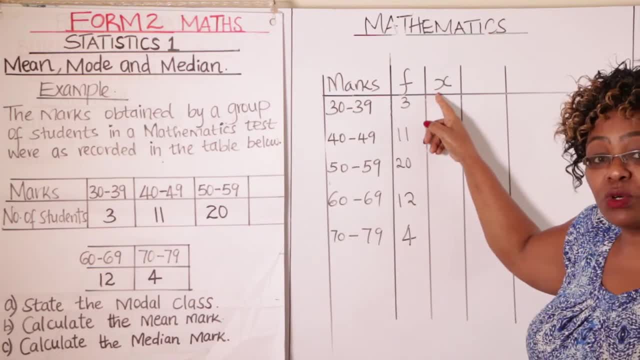 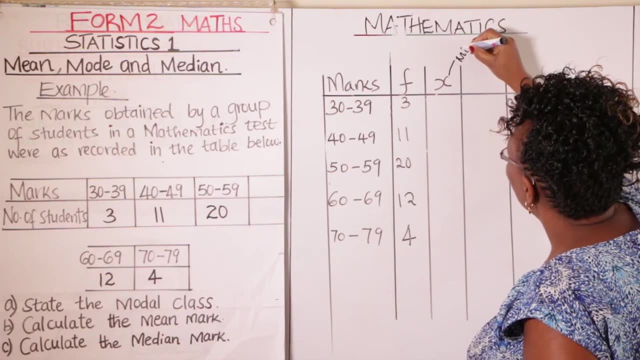 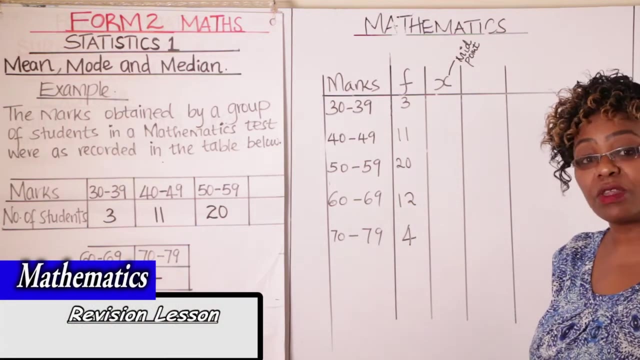 Here Tandem S crest Tandem. Then the third column. we put what we call x. What is your x? x refers to the midpoint of the classes. Midpoint x, lana, refers to the midpoint of the classes. 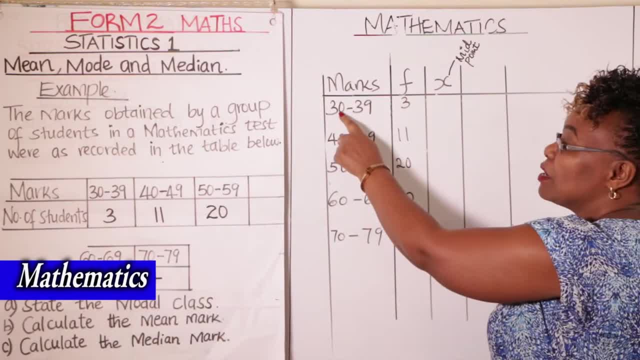 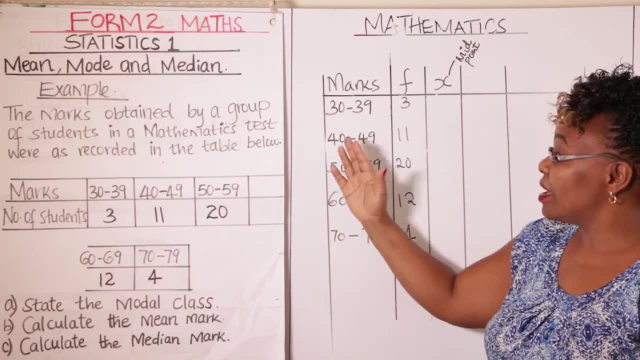 And therefore let us fill this column here. How do you get the midpoint of this class 30 to 39? lana? What you do? you don't need to write the numbers. There is a shortcut, and that is. it is a matter of adding this plus this: 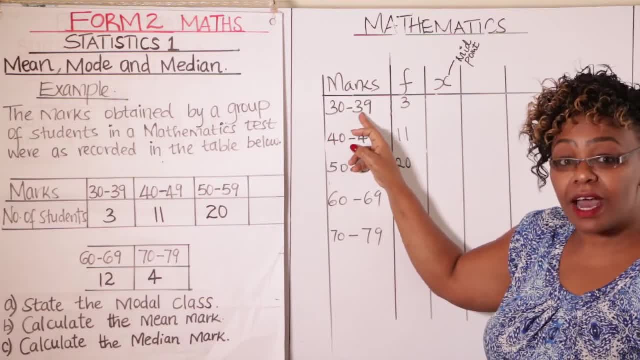 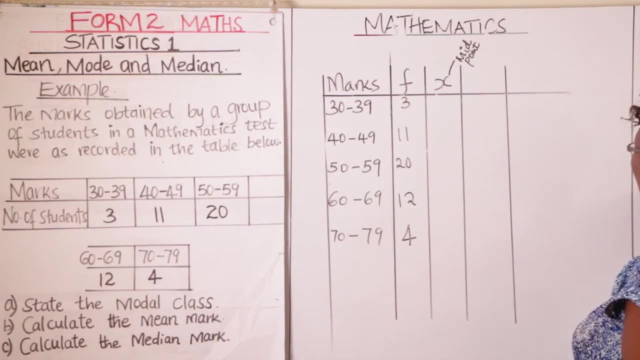 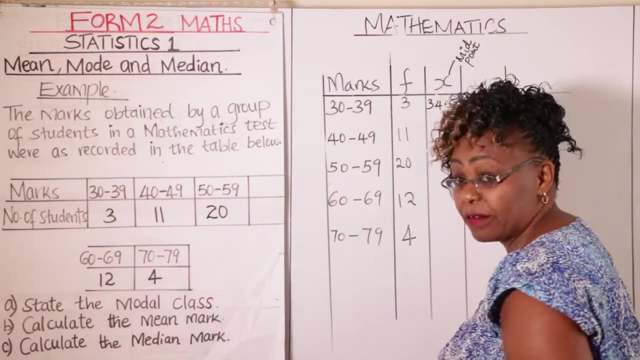 Then you divide by 2.. So 30 plus 39 gives you 69.. 69 divided by 2.. 69 divided by 2 would give you 34.5.. You come and put it here: 34.5.. 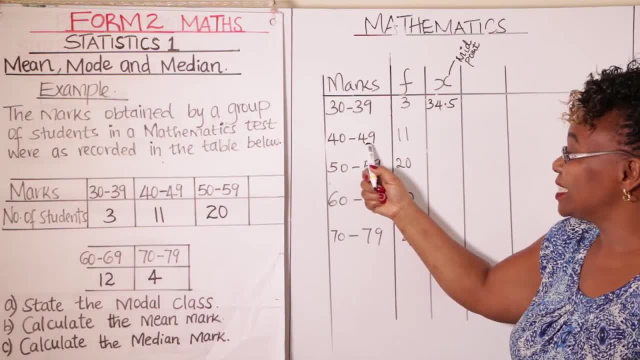 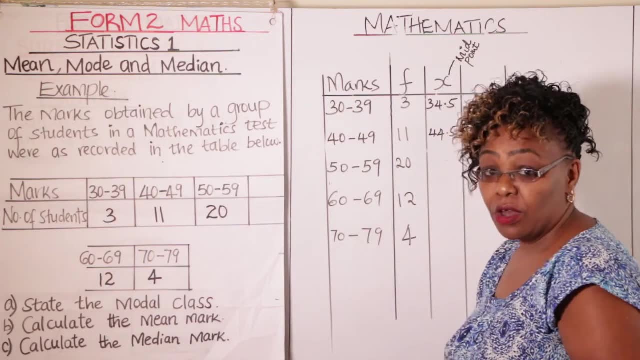 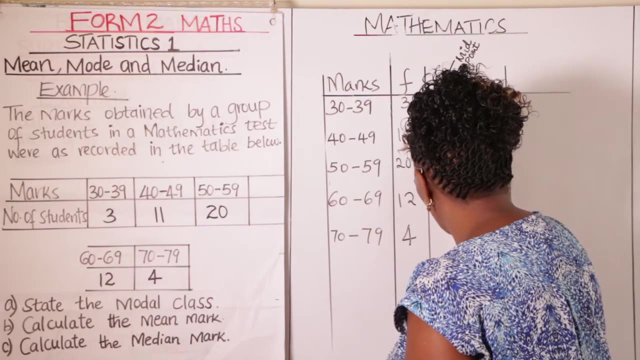 You add these two to get the midpoint. That is, 89 divided by 2.. 89 divided by 2.. It will give you 44.5.. You move on, lana. This plus this will give you a 9.. 195 divided by 2 will give you 54.5.. 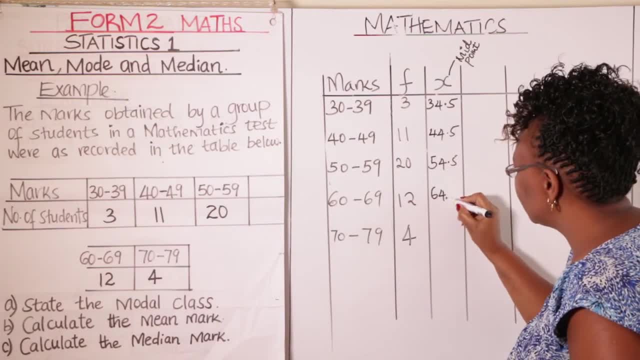 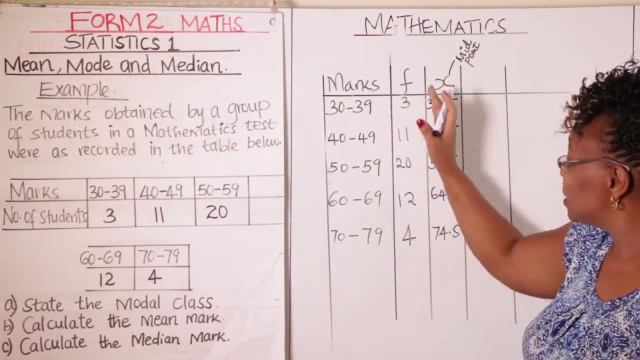 54.5.. You do the same here, You would get 64.5.. You would get here 74.5.. And therefore, lana, those are your x's, which refer to the midpoint. From there you come to the fourth column. 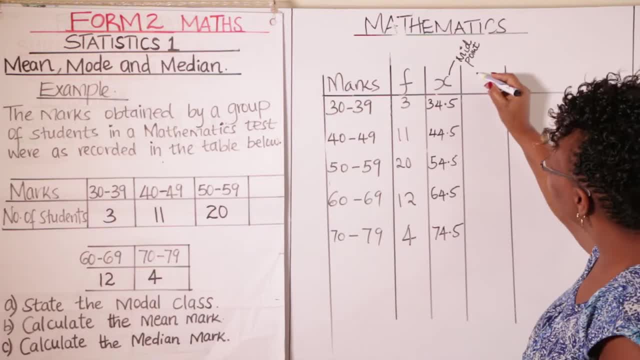 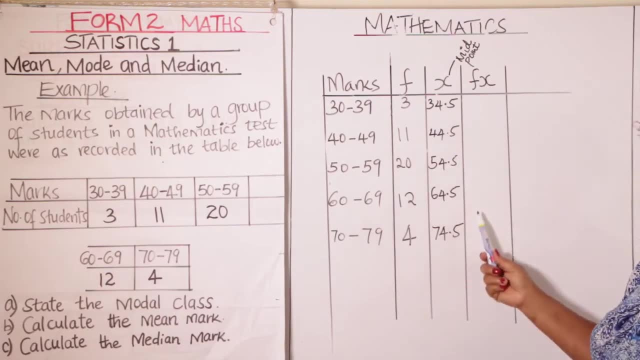 Here, lana, You come to the fourth column. You write fx f times x, fx. So in this column, to fill this column, you multiply your f times x, Your f times x. So, lana, you multiply this times this. 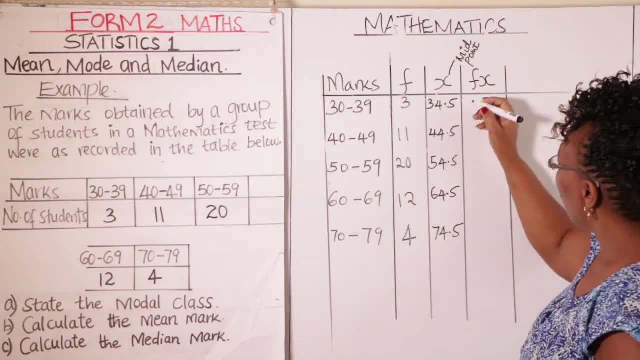 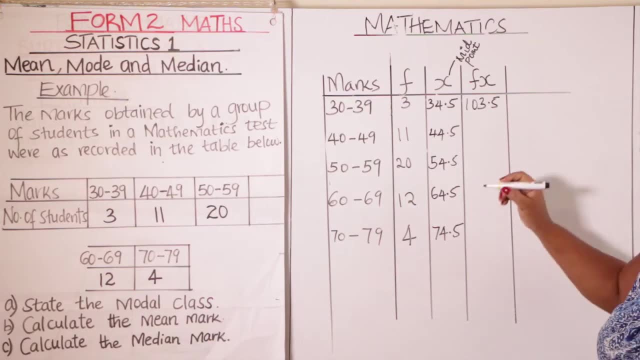 That 4.5 times 3 would give you 103.5.. Okay, You continue using a calculator there, You would get 489.5.. Multiply this by this, You would get 1090.. So, lana, you fill in that column of fx. 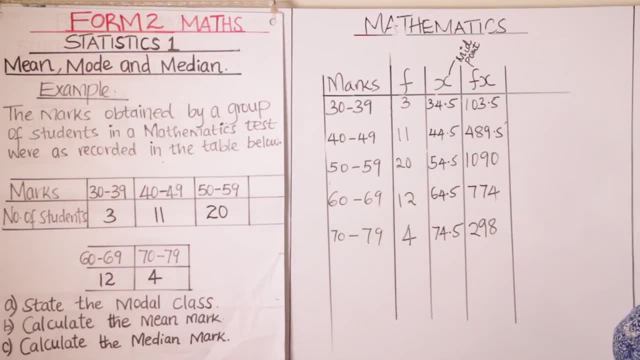 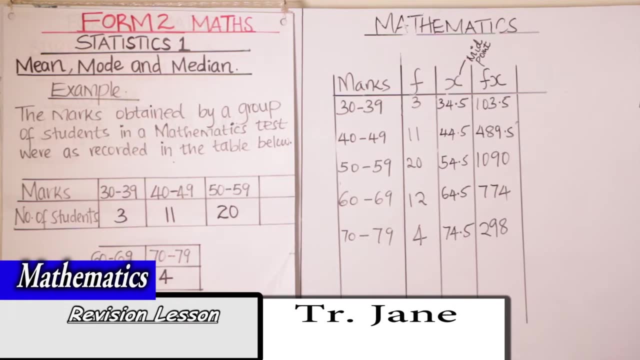 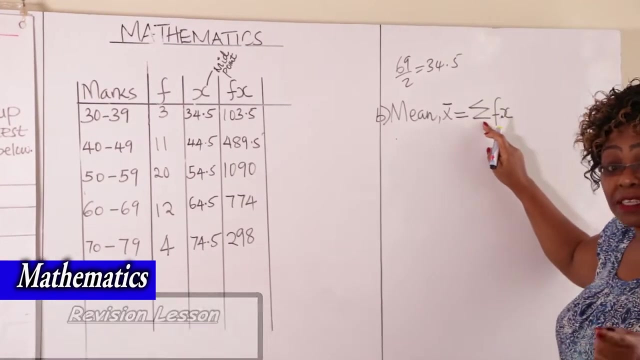 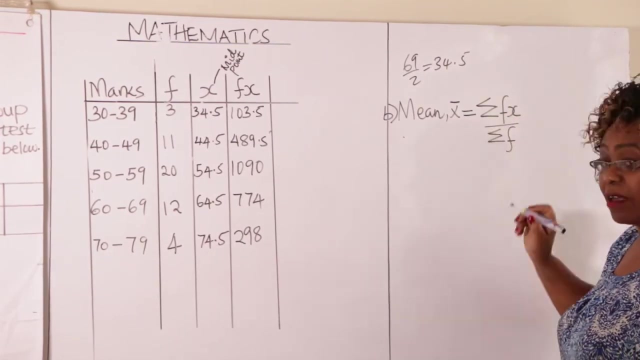 Multiply f times x, f times x. From there lana, the mean, which is symbolized as x bar, is given by formula, summation or sum, Sum, Sum of fx. You add all the fx's. This symbol means you add sum of all the fx's divided by the sum of f. 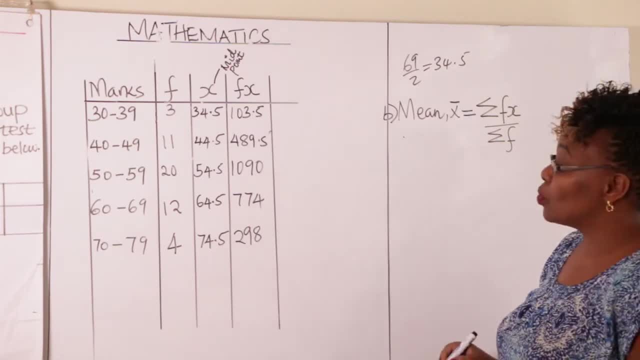 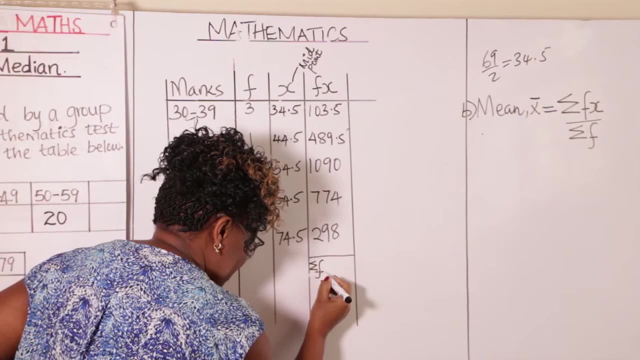 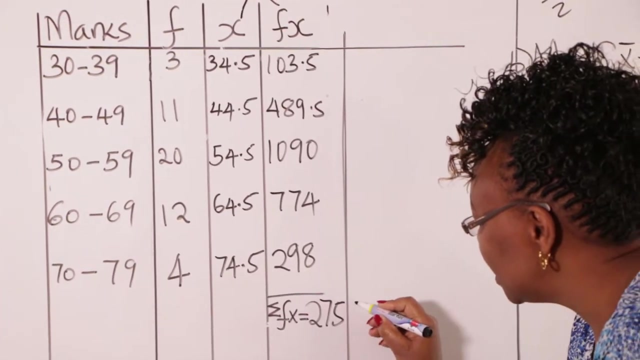 Divided by the sum of f. So, lana, you come and add all these fx's, So you come and write: sum of fx is equal to what You should get, 2750.. You then come and get the sum of f. 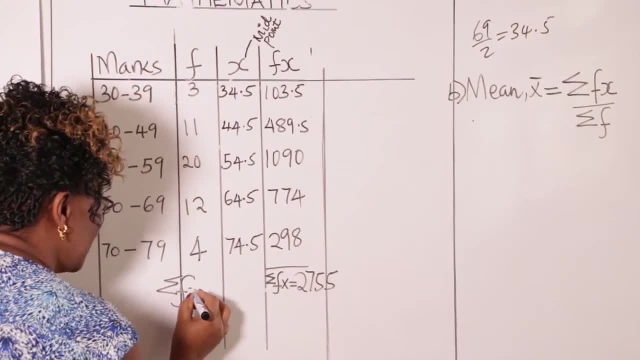 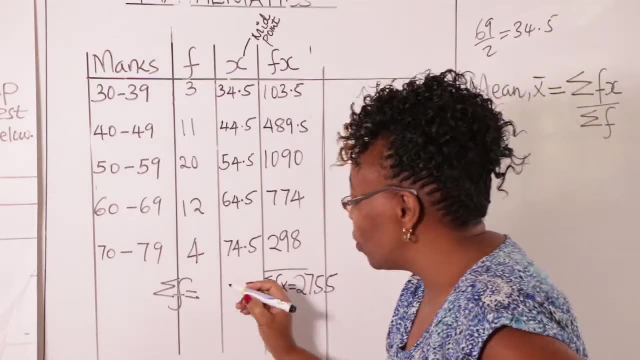 What would be your sum of f? here? I can write it here, Your sum of f. You add these frequencies, lana. Add the frequencies, You would get what You would get: 50. You are dealing with 50 students. 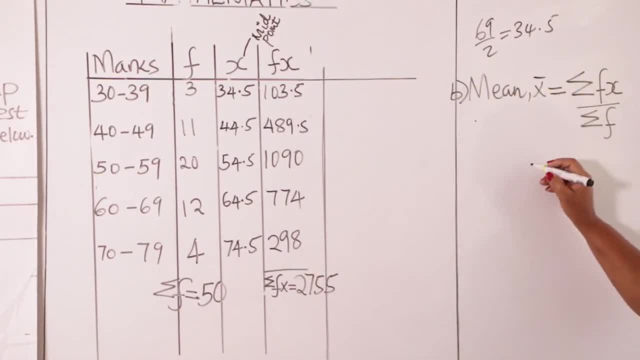 50 students. And therefore you come here and say: therefore, your mean will be equal to what, It will be equal to sum of fx, which is 2750.. And 55,, yes, divided by what? Divided by 50.. 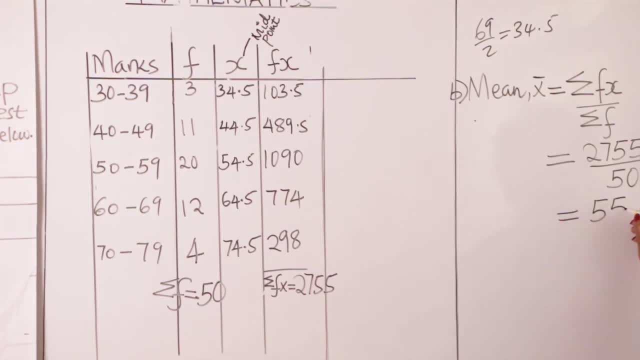 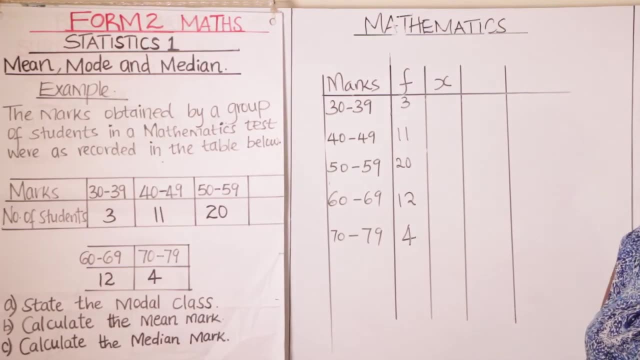 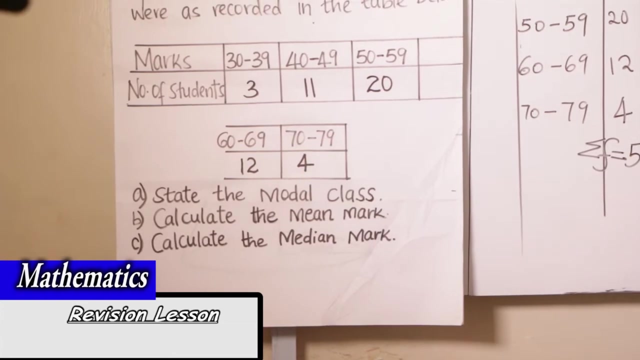 You work out that your mean should be 55.1.. That is the mean mark. So, lana, we go to part C, Part C of our question: Calculate the median mark, Calculate the median mark. So how do we go about that? 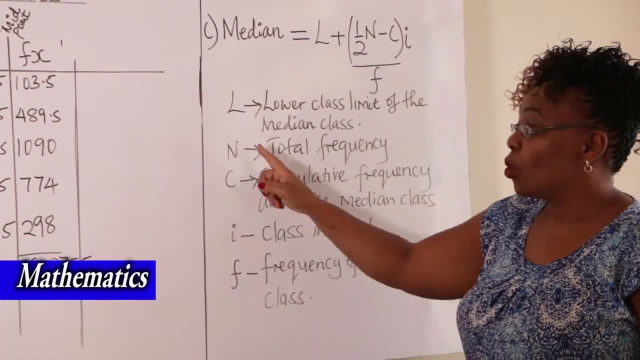 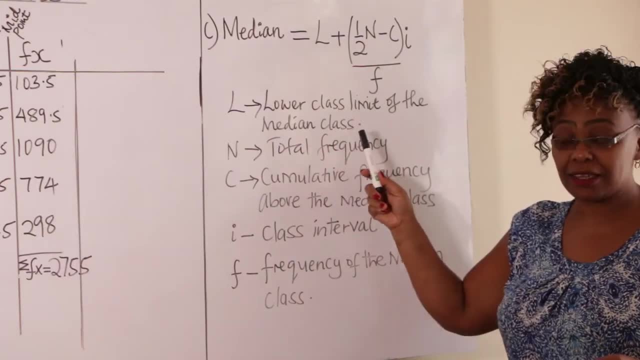 That is the formula for finding the median, Where l refers to what L lana refers to: the lower class limit of the median class. Lower class limit of the median class. We are going to see that C refers to cumulative frequency. 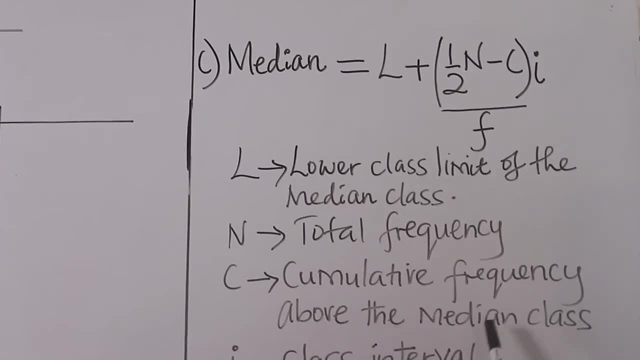 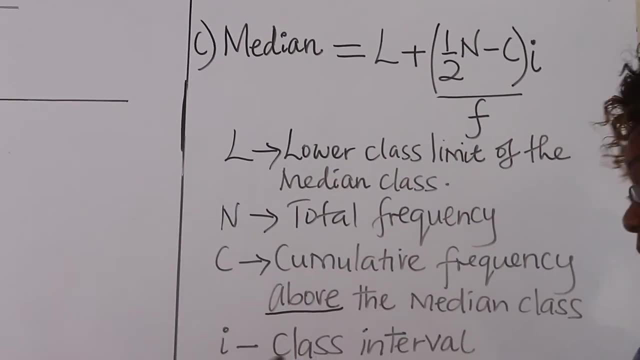 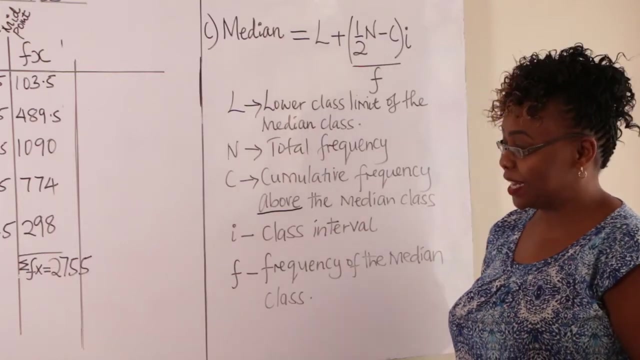 Cumulative frequency just above the median class. Above- We are going to look at this- Above the median class I. lana refers to class interval And f refers to the frequency of the median class. Frequency of the median class. 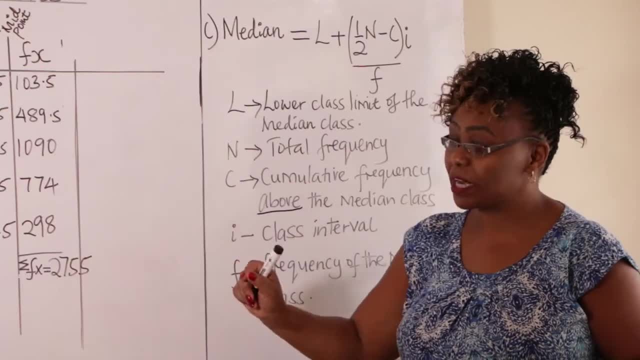 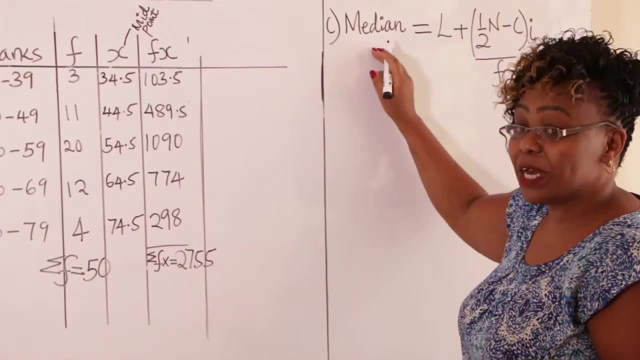 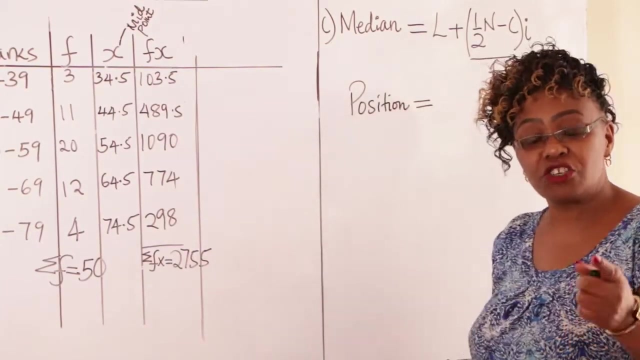 Good. So, lana, let us apply this in working out the median. So let us calculate our median now, lana, So our median. to get our median, you first identify the position of the median, Its position. Position of the median. 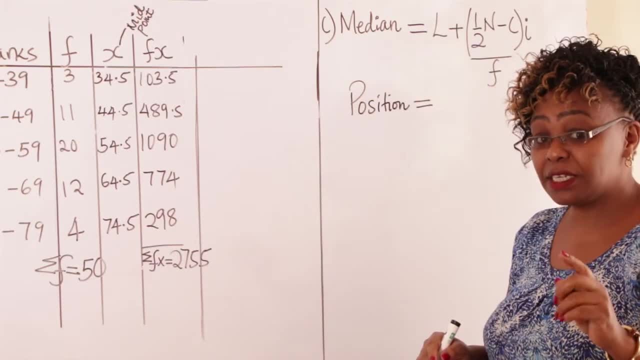 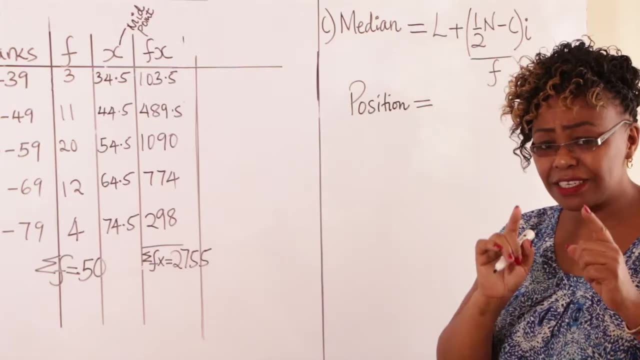 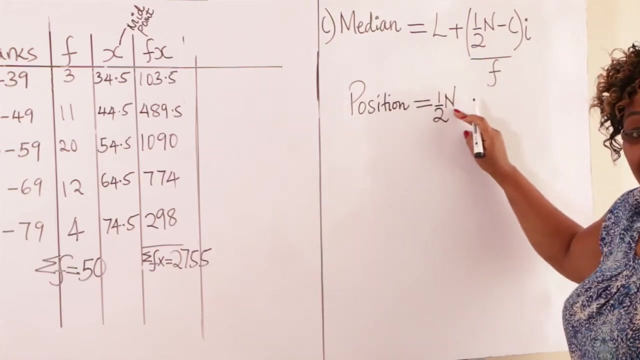 We have said that median is the value. It is the value that falls at the middle of a set of data. When the data is arranged in a setting, It falls at the middle And therefore it falls halfway the data. So it is a half of n, where n is referring to the total frequency. 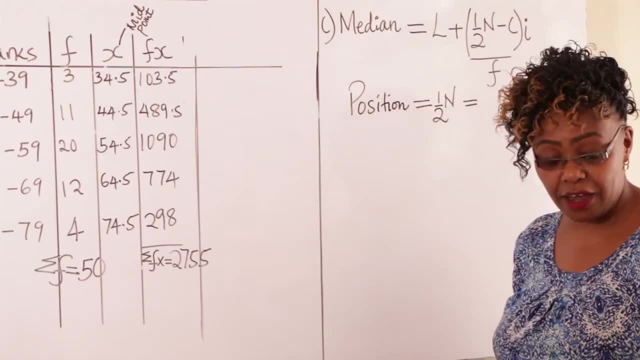 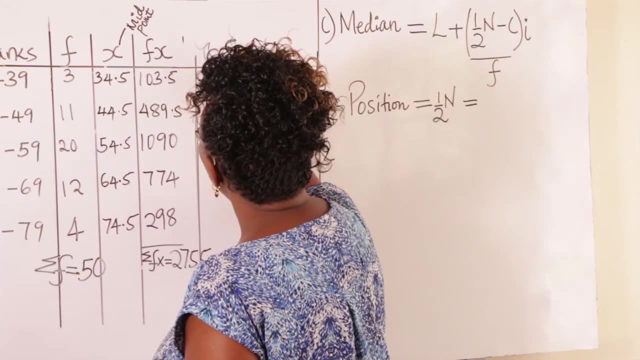 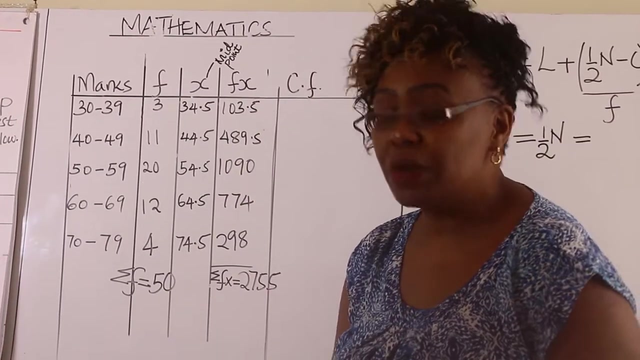 So, lana, where do we get? how do we get the n? To get the n, you go to your table and you add a column for what we call cumulative frequency. Maybe I can just write the symbols: Cumulative frequency. How do you get the cumulative frequency column, lana? 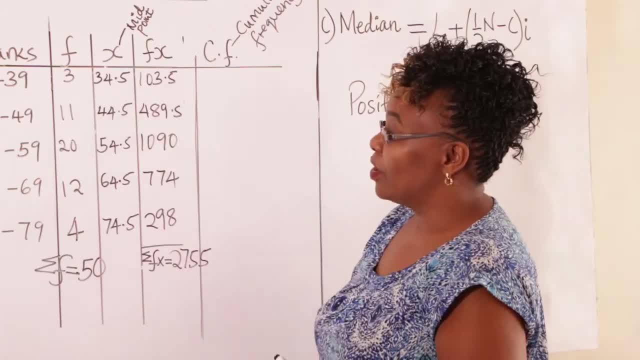 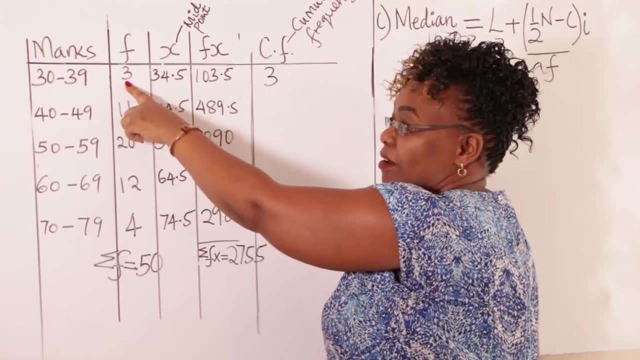 So how do you get the first cumulative frequency, lana? You come to your frequency column. This is 3.. You come and write the first value there of the frequency. From there to get the second one, you say 3 plus the next. 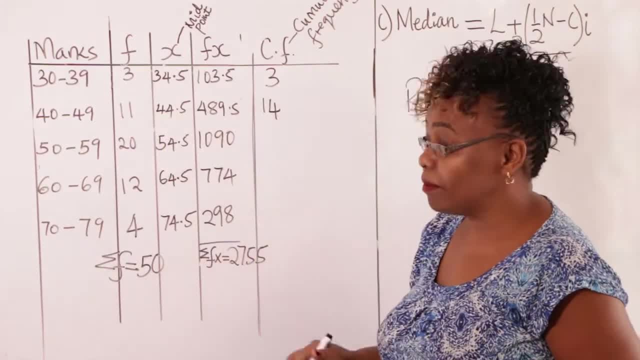 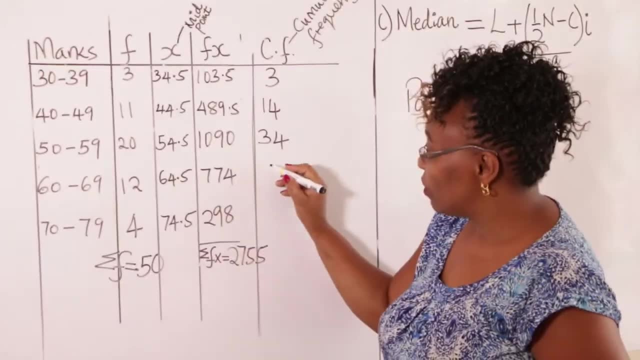 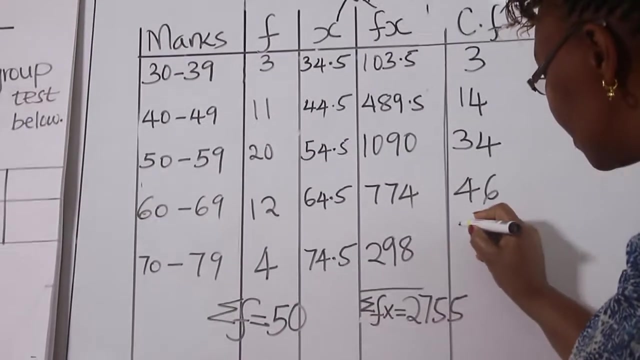 3 plus 11 gives you 14.. Okay, 14 plus 20 gives you 34.. 34 plus 12 gives you what? 46.. Okay, 46 plus 4,, lana, the last one gives you 50.. 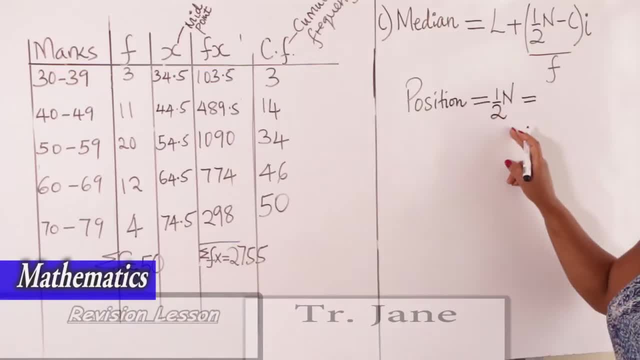 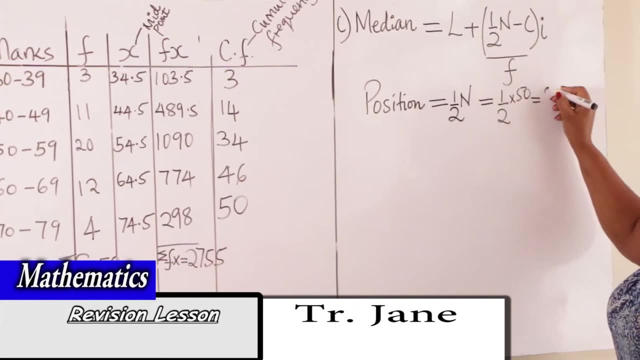 So we are dealing with 50 students And therefore we come back to here: So our n is 50. And therefore we come here and say this is a half times 50, which gives you 25.. So our median lies on the 25th position. 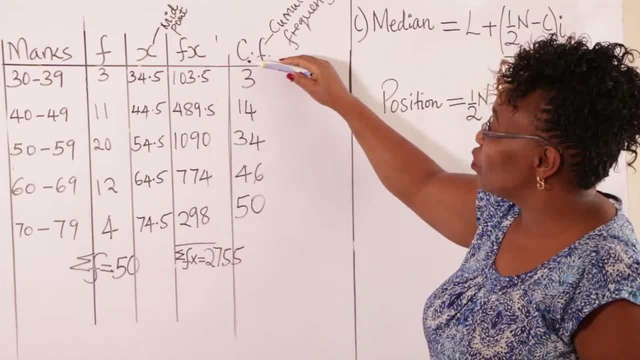 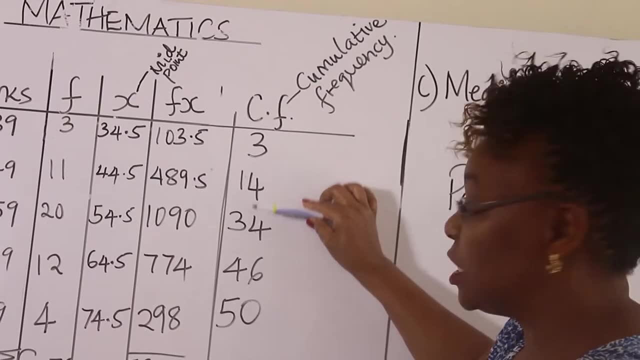 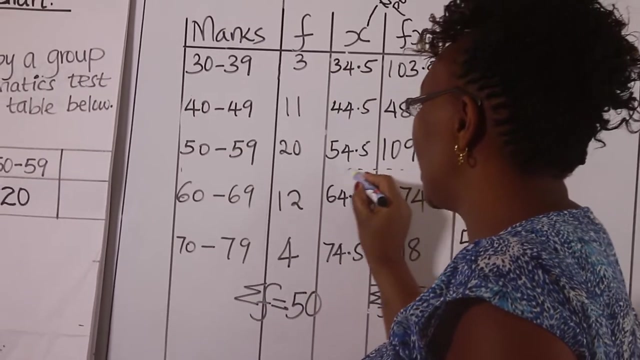 So you come to that. So our median lies on the 25th position. So you come to that. So you come to that frequency, I mean cumulative frequency column. you check where your 25 will lie: 25 this is 3, this is 14. so 25 lies here. it lies here. you come and mark that row. 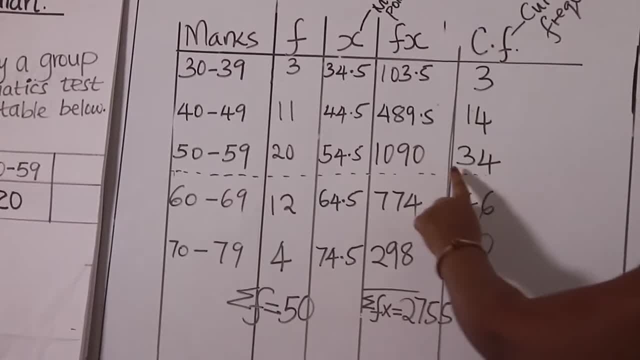 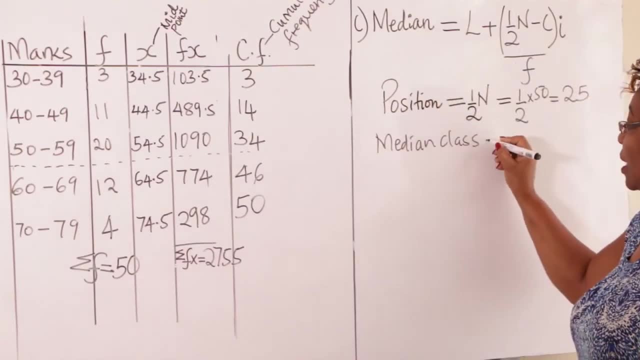 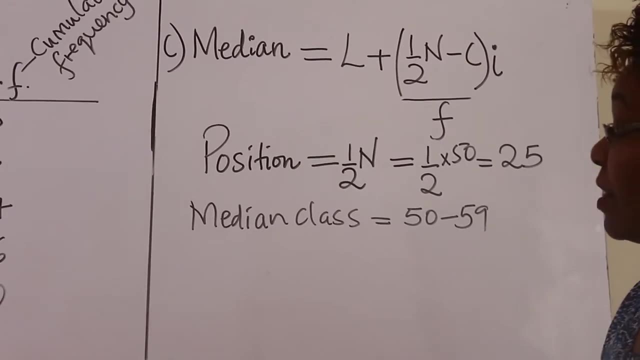 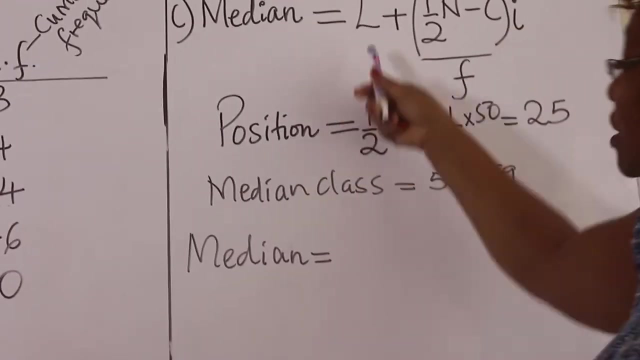 like that and therefore your median class. you come and write that your median class is 50 to 59, your median classes fifty to 59 and they are for lan. you now come and see your median is what. therefore, you get your L in lower class limit of the median class. how do you get it? you come 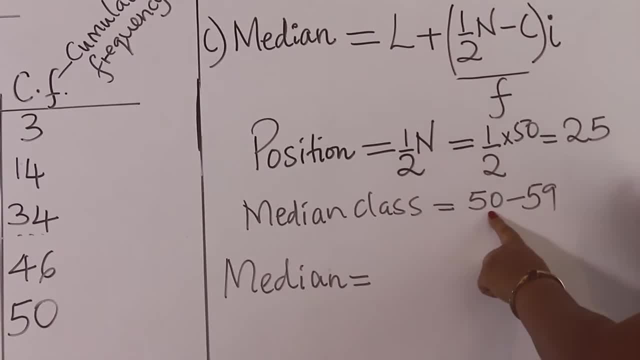 to the lower number here: 50. you subtract 0.5. 50. you subtract the 0.5. 50. you subtract the Zul from your class. Oh, you subtract 0.5, 50, you subtract 0.5 and get it. we drop the straightlyás 5, even hackers. but now we know why the average is different. instead of the average class is 50. you express a class C, major Class duration, ski program. we get a certain number around theкрame class, history as well. you suspect I got to diag for 11, seven, leaving class here: 50. you subtract. but the engineering class, history class, history c, just before name of standing, does not in this class. you genius less of the psn physical class and you do so over the course. so you subtract what you remember it, yoga class rampage, and you get to this quarter. we have no case by tails. 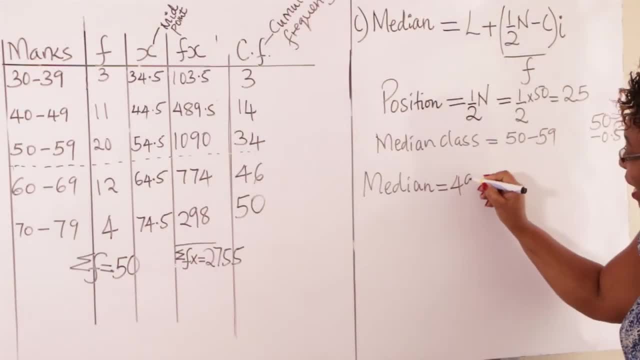 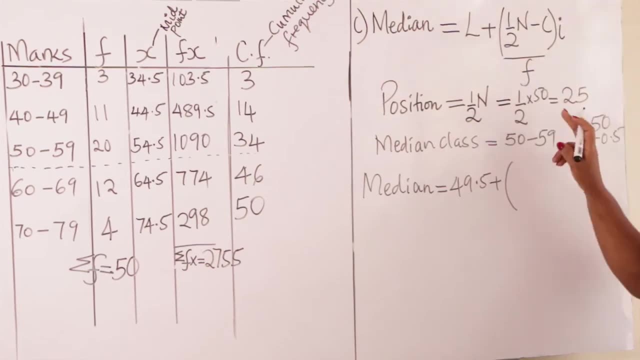 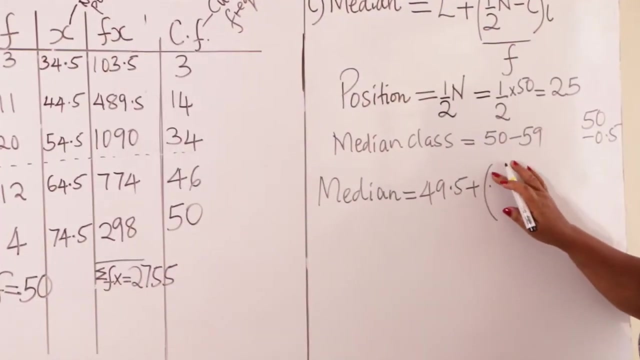 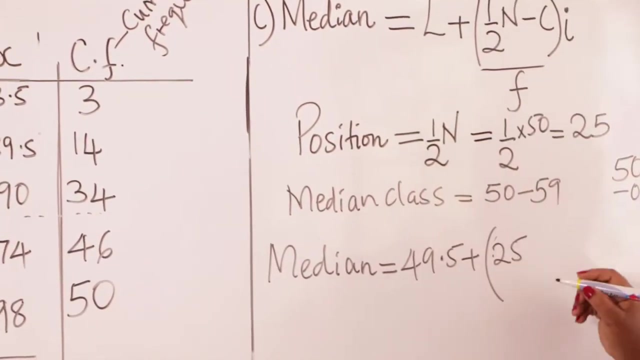 49.5 and therefore you get 49.5 plus bracket. A half of n, a half of n, We already have it. A half of n is 50. A half of n, So maybe you can write it. A half of n will give us 25. Direct 25.. A half of n, We have already got it. 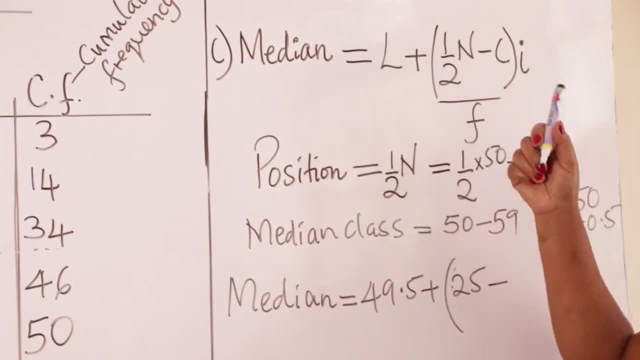 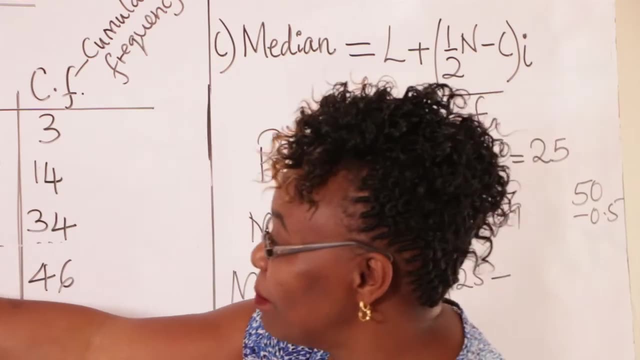 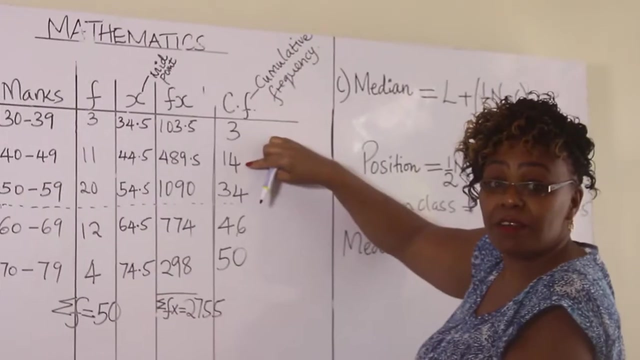 Then minus what Our c C refers to the cumulative frequency just above the median class. So you come here. This is our median class. This is the row that we mark, Which is the cumulative frequency above this. It is 14. 14.. So come and write 14 there. 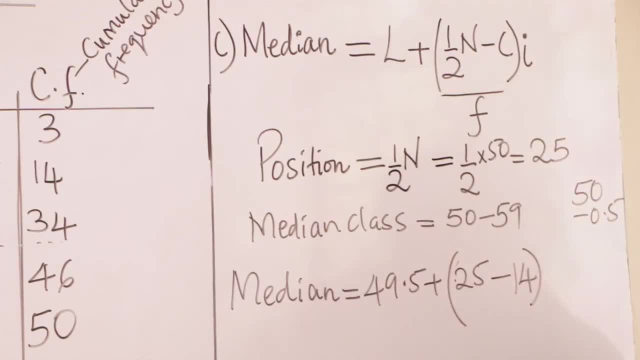 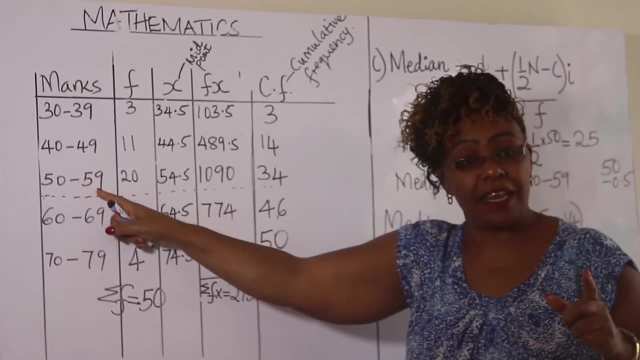 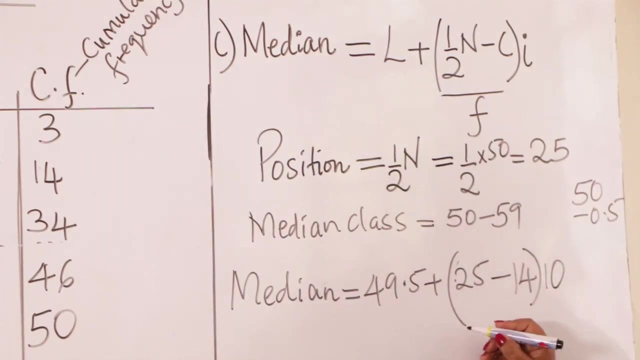 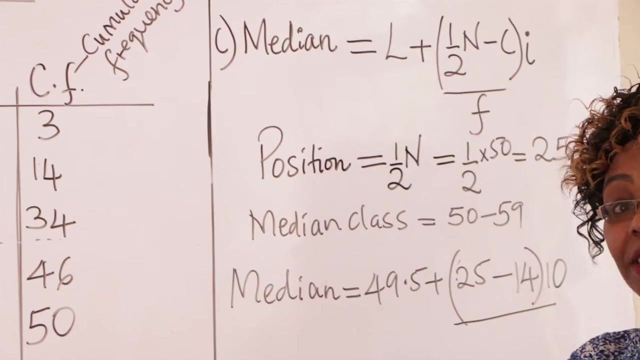 Multiply by i. I learner. we have said it refers to. It refers to the class Interval From 50 to 59. How many values are those? Those are 10. 10. So you come and write your 10 there, Unified by f. F means what? Remember what we said: F refers to the frequency of the median class.